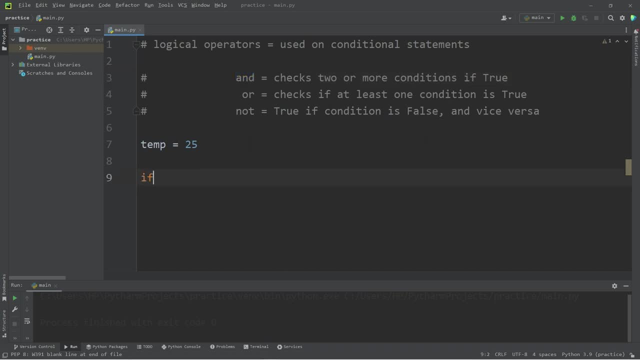 Let's check if our temperature falls between the range of between 0 and 30. If TEMP is greater than 0 and TEMP is less than 30, then we will print: the temperature is good. If this condition is true- and this condition is true, then we will execute this code. Else, we will print. 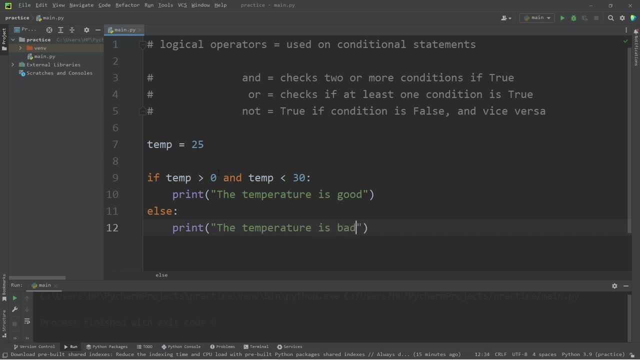 the temperature is bad. Our temp is currently 25.. The temperature is good. What if it was negative 10 degrees Celsius? Well, the temperature is bad. What if it was over 30,, like 40 degrees Celsius? Well then, the temperature is still bad. Using an AND logical operator, if one of these conditions: 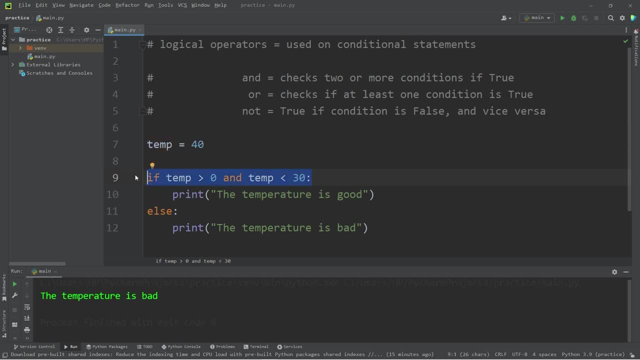 is false, then this entire statement will evaluate to be false. We would then skip over any subcode and continue on. Using the AND logical operator is pretty convenient. if you need to check to see if something is within a certain range, like a temperature, There is another way we can write. 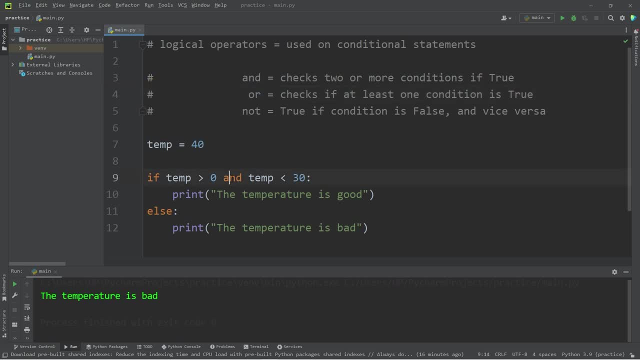 this, too, using the OR logical operator. Let's replace AND with OR. Let's replace AND with OR. If at least one of these conditions is true, then the entire statement is true. How about if TEMP is less than or equal to 0, or if TEMP is greater than or equal to 30?? 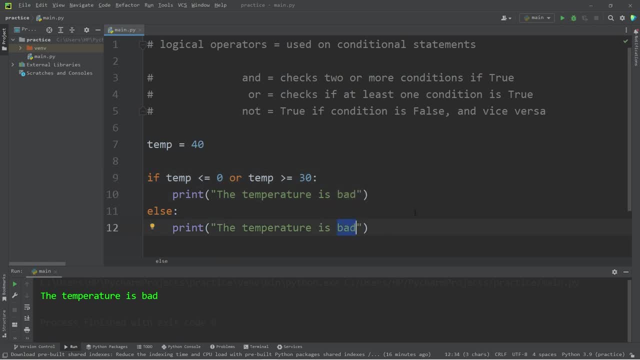 Then the temperature is bad. Else the temperature is good. Currently, our temperature is set to 40.. Well, the temperature is bad. This is false, but this is true Using the OR logical operator. only one of these conditions needs to be true. If our temperature was negative 15,. 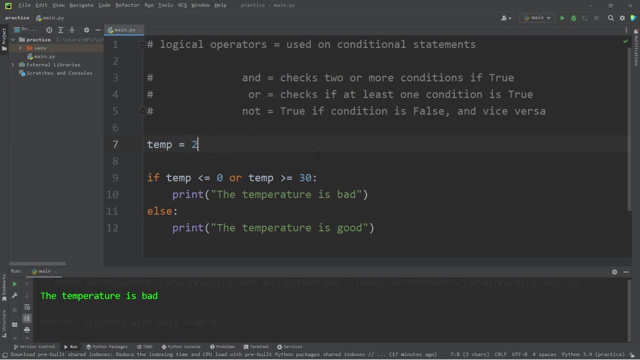 well, the temperature is still bad, But if it was 20,, well then, the temperature is good. AND as well as. OR are fairly similar With AND. two or more conditions need to be true. for the statement to be true With OR, only one of them needs to be true. Is this true or is this true?